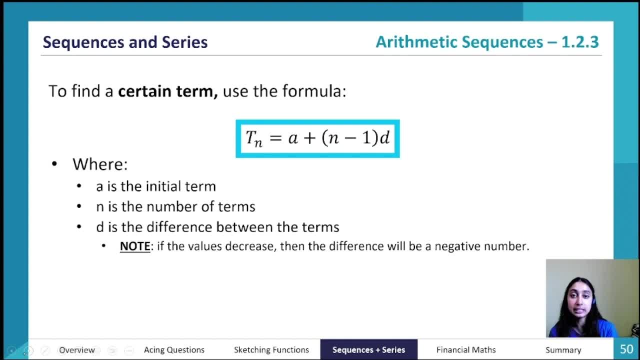 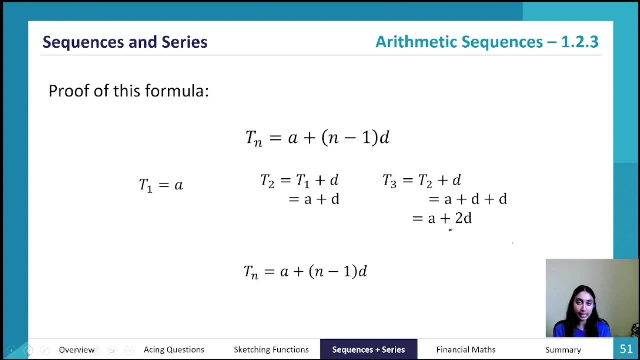 A, as I was saying before, is the first term, n is the number of terms, so the nth term, And then d is the common difference between the terms. Yeah, And then we're just going to prove that formula to you. So if we know that A. 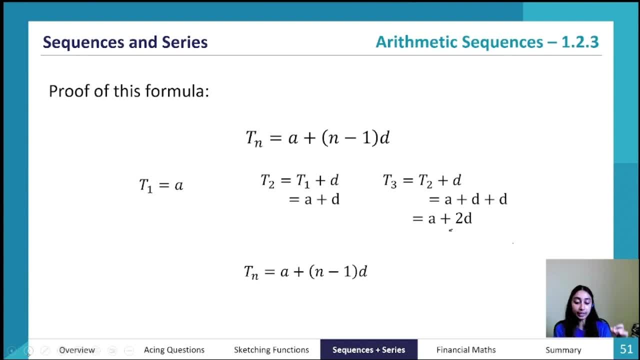 is T1, then T2 will be T1 plus whatever the common difference is. so A plus d, T3 will be T2 plus d again, So A plus d plus d, So A plus 2d, Which, if you just keep going into- 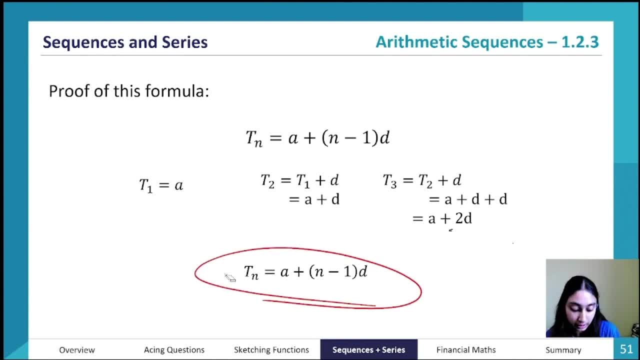 whatever n, you'll still be boiled down to the same formula. Tn is equal to A plus n minus 2jn. Okay, so that's also on your formula sheet, by the way. With this in mind, let's try this question. 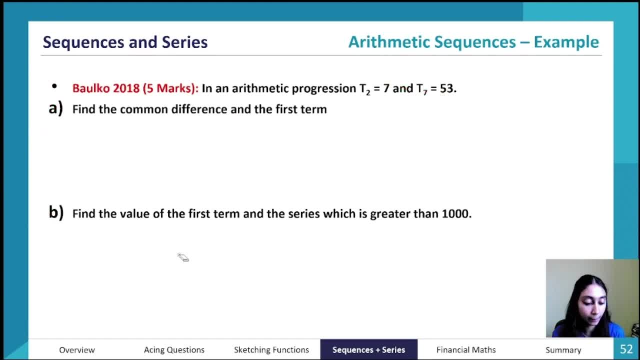 I'm not going to give you any time to go through it on your own, so you can pause. if you'd like to go through this, Okay so Bochum Hills 2018.. In arithmetic's progression, T2 is equal to 7,. T7 is equal to 53. 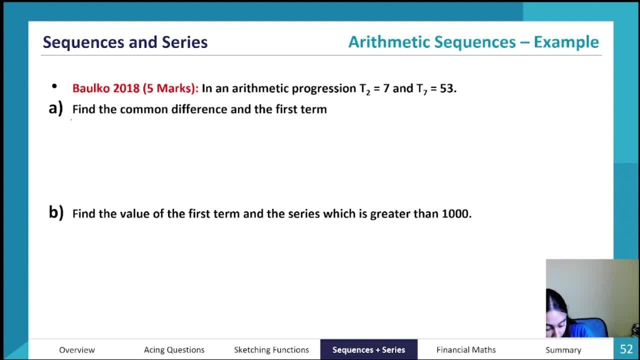 Find the common difference in the first term. Okay, so I'm going to write the equation at the top. So Tn is equal to a plus n minus 1d. T2 is equal to a plus 2 minus 1,, which is 1, times d. 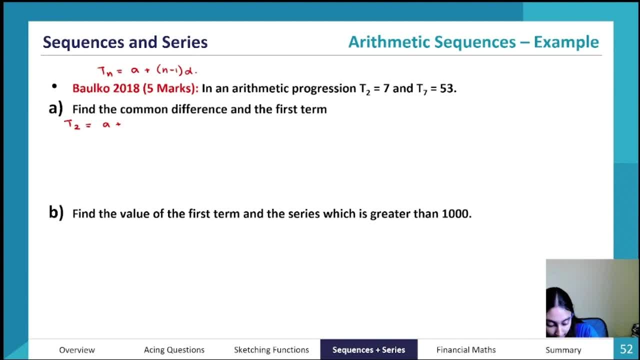 Okay, so I can write that a plus d is equal to 7.. Okay, what else can I write? I can write that T7 is equal to a. T7 is equal to a plus 7 minus 1, so 6d, which is equal to 53.. 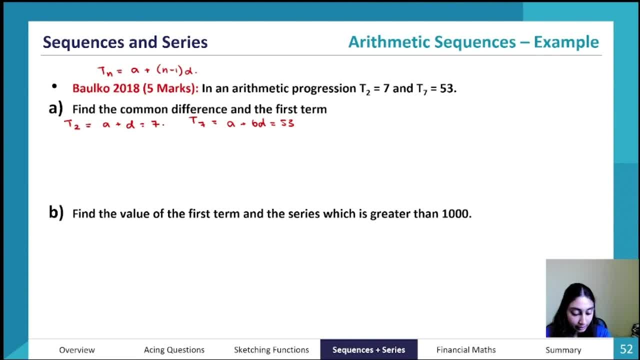 So what I'm going to do is I'm going to – I mean, you can choose what you'd like to do with this. You're going to have to do simultaneous equations. I'm going to define d, Actually, no, I'm going to define a. 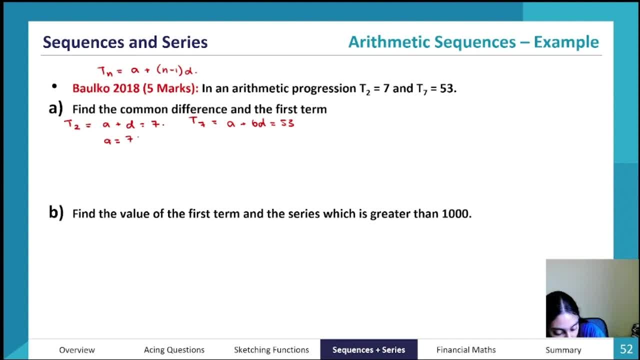 You can pick, It won't make a difference. So a, a is equal to 7 minus d. okay, So now I'm going to sub a is – well, basically sub 1 into 2.. So T7 is equal to 7 minus d, plus 6d is equal to 53.. 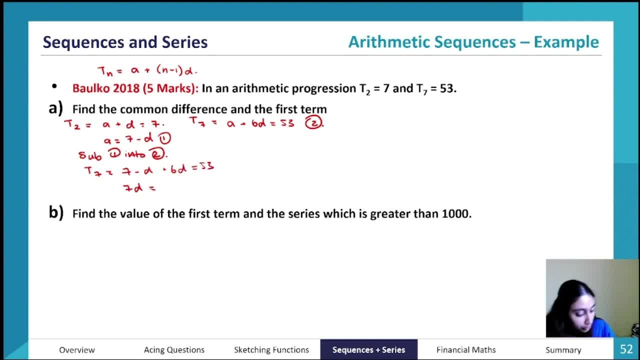 Okay, 7d. 5d is equal to – oh, not 7. Sorry. 5d, 53 minus 7. 46.. So d is equal to 46 on 5. 9.2. Okay. 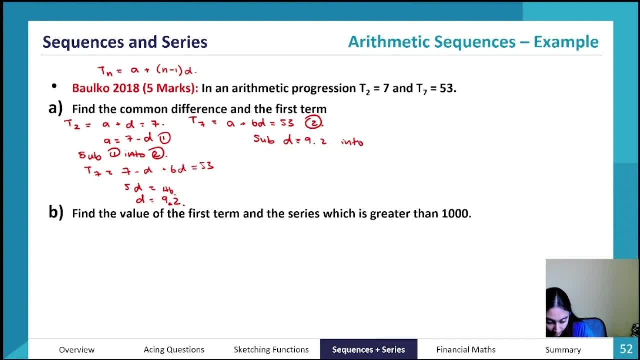 Sub d is equal to 9.2, into the first equation. So a is equal to 7 minus 9.2, which is negative 2.2.. Okay, And now my next step is to obviously check. So check by subbing into a: 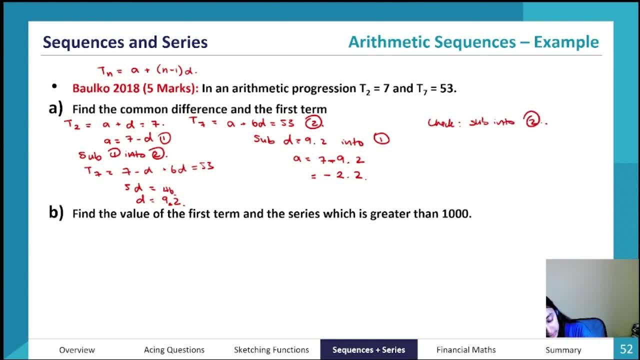 Oh sorry, 2.. So I get minus 2.2 plus 6 times 9.2.. All right, So my plus 7 plus 2 times 9.2 is equal to 53, which is correct. So my a and my d. 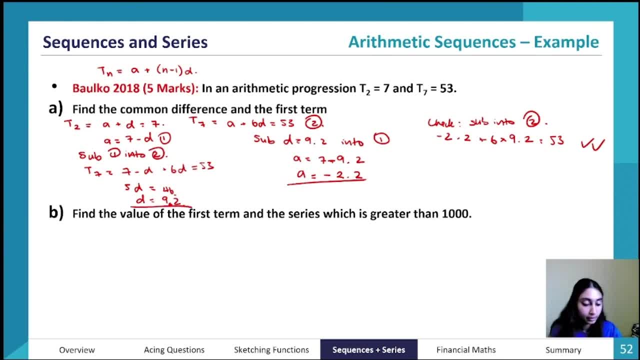 Okay, The next question is to find the value of the first term and the series which is greater than 1,000,. okay, So let's do – okay, let's see, Let's call it 50.. Let's make some calculations here. 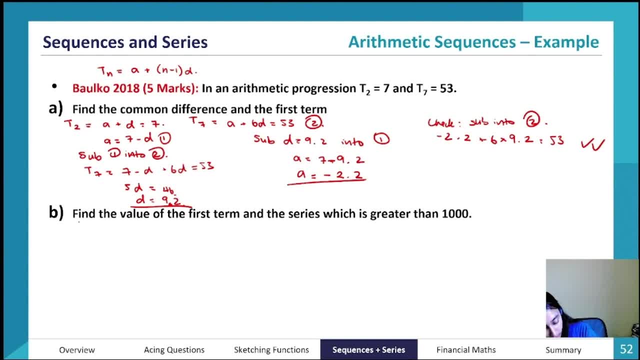 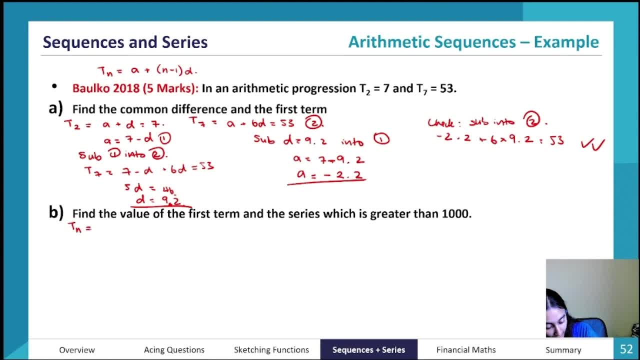 Okay, Let's see. the actual equation for Tn is equal to a, so negative 2.2 plus n minus 1 times 9.2.. I'm actually going to expand these brackets, so it's going to get me to minus 2.2 plus 9.2n minus 9.2,. 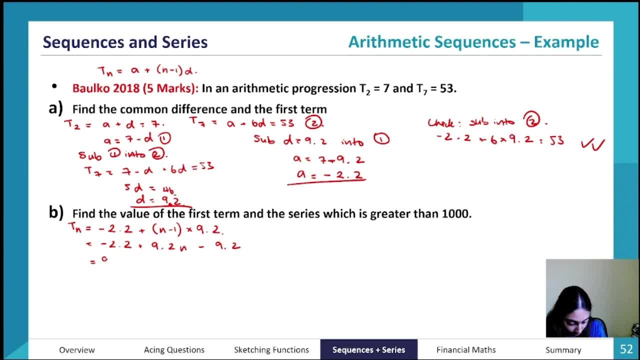 which will get me to 9.2n minus 11.4 is equal to Tn. okay, So I'm looking for the term value that'll be greater than 1,000.. So I'm going to say that 1,000 is equal to 9.2n minus 11.4.. 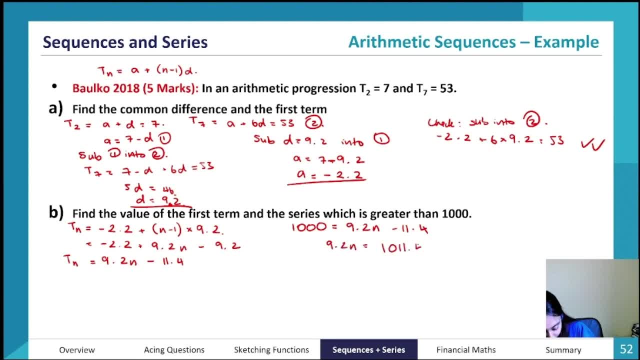 9.2n is equal to 1,011.4.. n will be equal to 1,011.4 divided by 9.2,, which will be 109.93,. blah, blah blah. So my next thing is to check what the question is actually asking for. 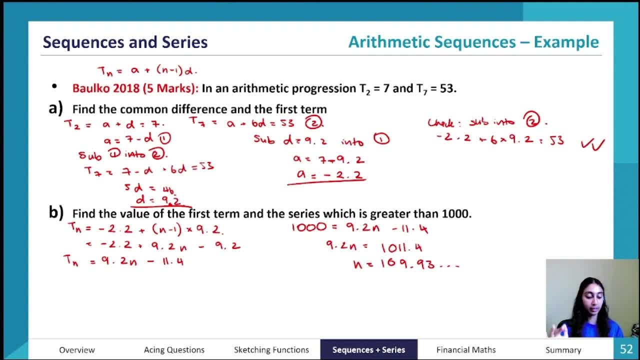 Is the question asking for what's greater than 1,000? So I'm going to sub in 109 into my Tn. 109 will get me 9.2 times 109 minus 11.4.. That gets me to 991.. 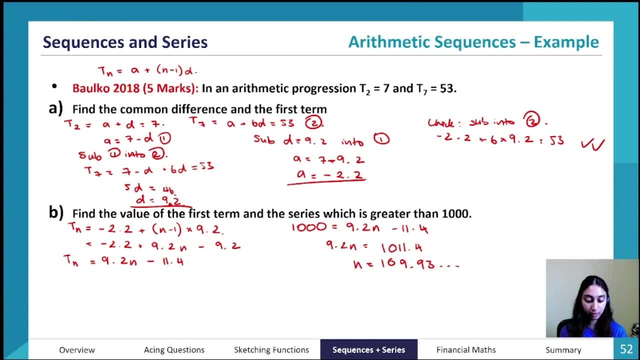 We're not there yet. We're not over 1,000.. So if I go to 110, I should be, yeah, 1,006,. okay, So therefore, n is equal to 110, but that's not answering my question. 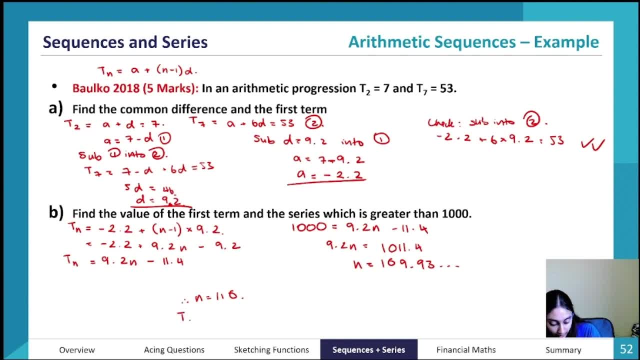 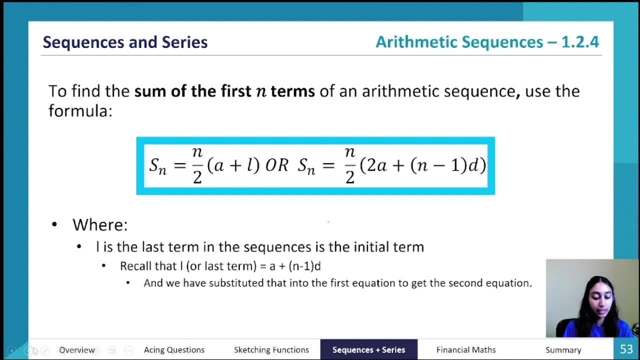 The question wants me to know. the value of the first term, T110, is equal to 1,000.6, and that's how we answer this question. Awesome. Let's move on to the sum of the n terms which is given by these equations. 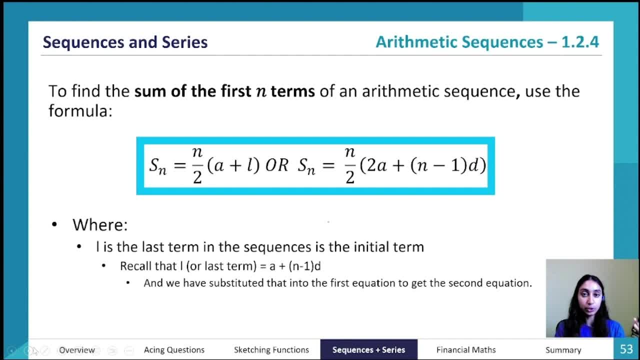 also given on your formula sheet. So Sn is equal to the number of terms on 2 times a plus l. so the first term plus the last term, which is proven in a really cool way. I'll show it to you in the next slide. 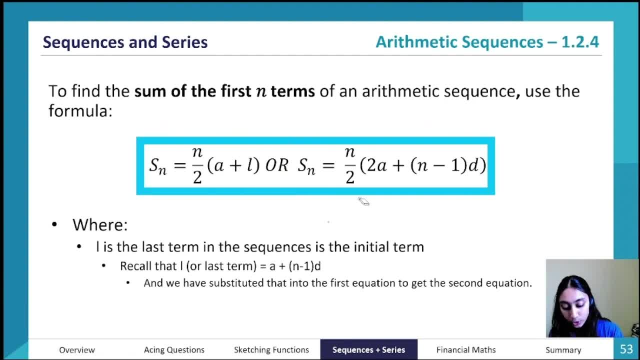 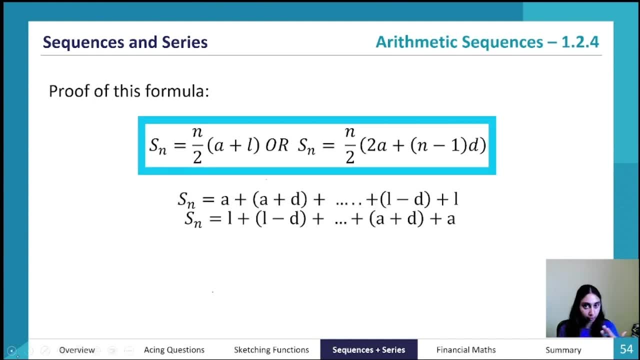 And from this equation we can derive this equation, which is also given In the formula sheet. okay, So the way that this formula was derived is: there was this German mathematician which I can't remember his name, but he pretty much just defined the sum. 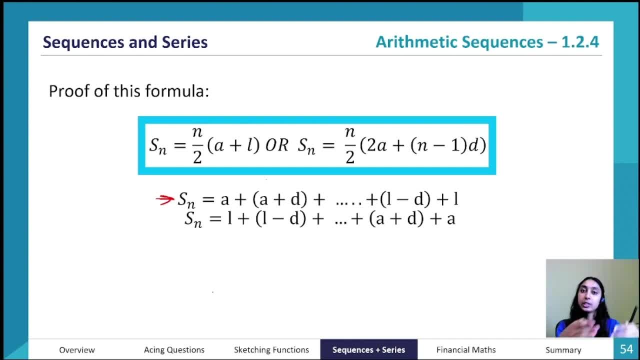 of n numbers, to be term 1 plus term 2 plus term 3 plus term 4 plus blah, blah, blah, which will be, You know, a plus a plus d plus a plus d plus d, and so on, so on, so forth. 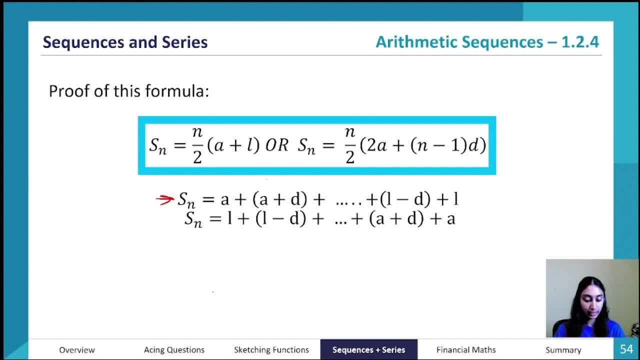 And then, obviously, because they're all being added, if you just flip them over, it'll be the same thing, And then, when you add these together- so 2 Sn- you'll find that everything cancels with each other, except for our a plus l. 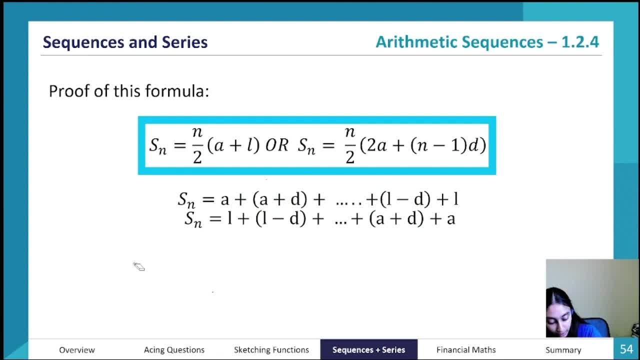 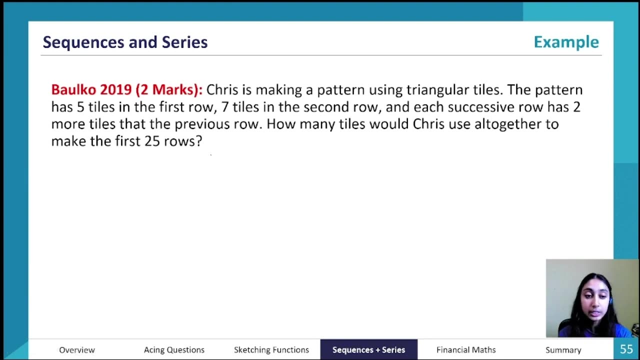 So you're left with just: Sn is equal to n and 2 times a plus l, so that's a pretty cool formula. Okay, so we have a question also from: Chris is making a pattern using triangular tiles. The pattern has five tiles in the first row, seven tiles in the second row and each successive. 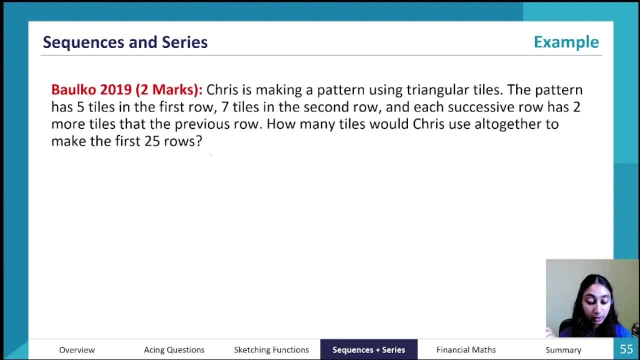 row has two more tiles than the previous. Okay, How many tiles would Chris use altogether to make his first 25 tiles? I'll give you a sec to pause this question and work through this on your own, okay. Okay, hopefully you have done the question now and I'm going to show you the working. 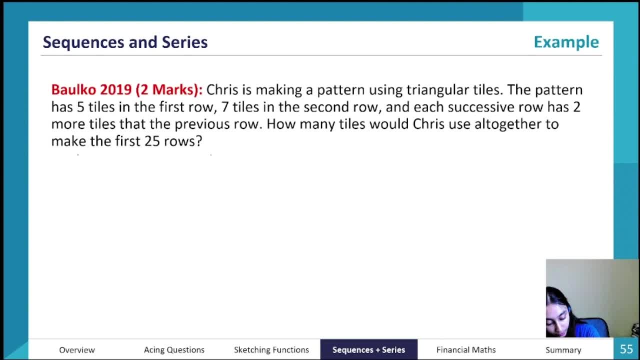 Awesome. Okay, so the first tile, so T1, is equal to 5, and our common difference is equal to 2.. So Tn is equal to 5 plus n minus 1 times 2,, which is equal to 5 plus 2n minus 2.. 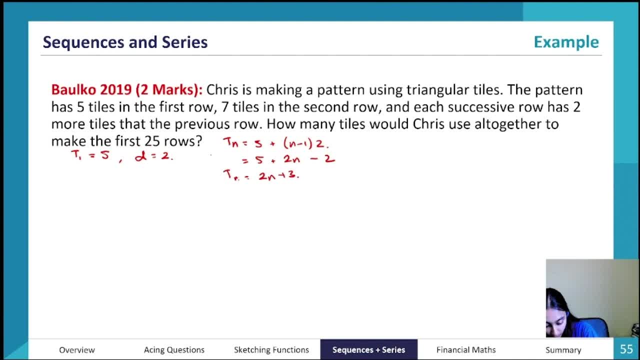 So it's equal to 2n plus 3, okay, Which I suppose I didn't even need to do, but I did it anyway. Okay, now we'll do the sum of 25.. So there's two ways that you could do the sum of 25.. 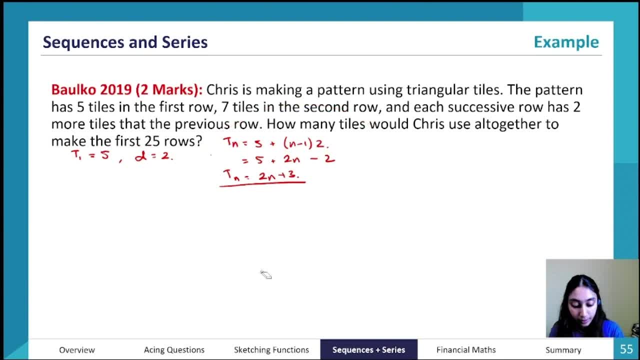 It could be first or second. Okay, So I'm just doing this and then doing the first equation, which is: Sn is equal to n on 2, a plus l, my personal favorite, but you'll need to know how to use both equations.